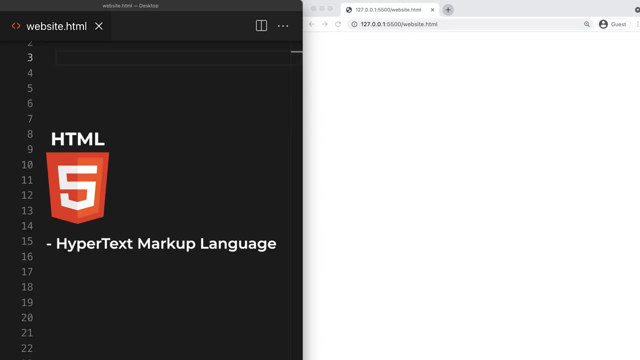 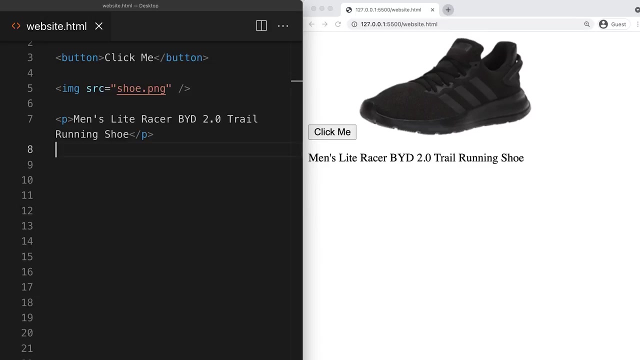 is HTML. HTML stands for hypertext markup language and is used to add content to our webpage. For example, I can write this bit of HTML to add a button. I can also add other types of content, like images and text, and if I write more HTML, 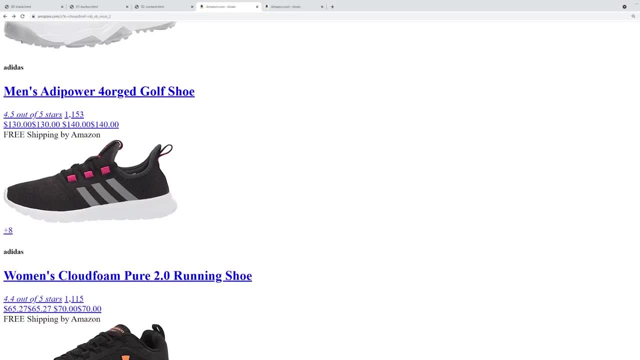 it will add more content to my page, But you'll notice that our page doesn't look very good. That's where CSS comes in. CSS stands for Cascading Style Sheets And, based on the name, it's used to style our webpage, So it's used to make our webpage look good by letting us adjust. 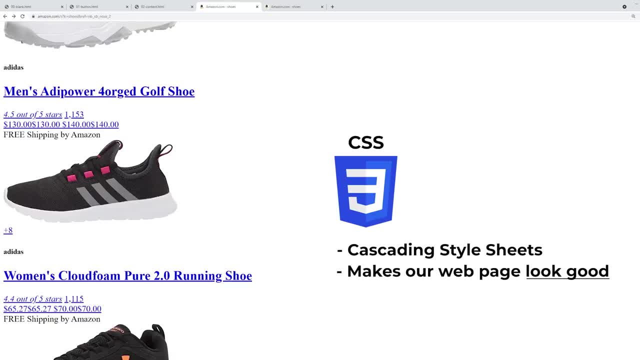 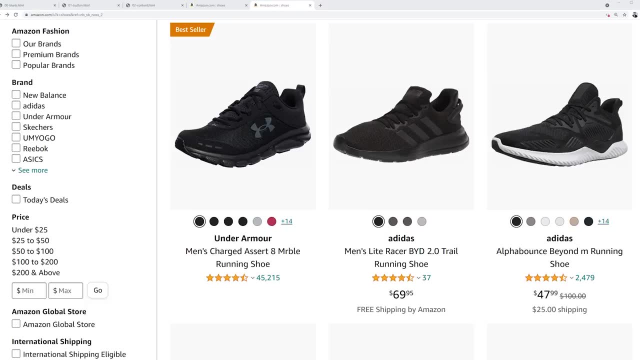 colors, sizes, spacing, things like that. Let's add some CSS to our page So now that looks much better, but we're not done here. Let's say that I want to filter these products and only show one brand of shoes, so I click this checkbox, But you'll notice that nothing. 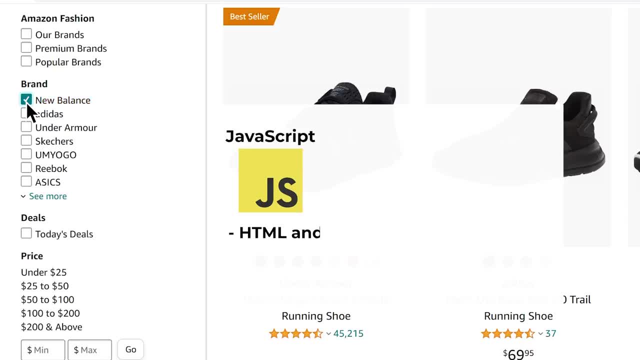 happens, And this is because I want to use CSS as a separate product and not just another brand of shoes. So I click this checkbox. And when I click this checkbox, I can see that I'm not seeing. anything is where javascript comes in. html and css only display things on our webpage, but javascript is. 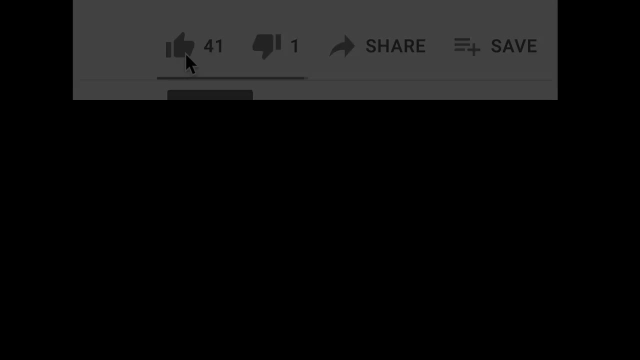 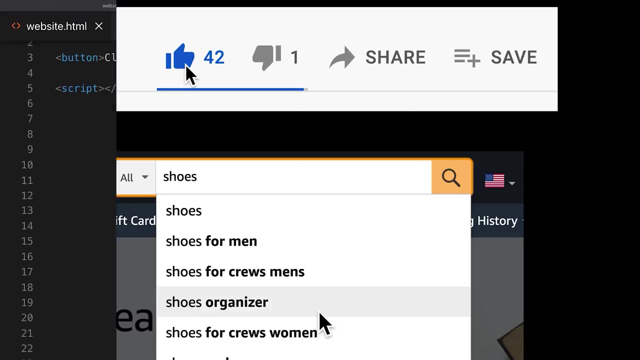 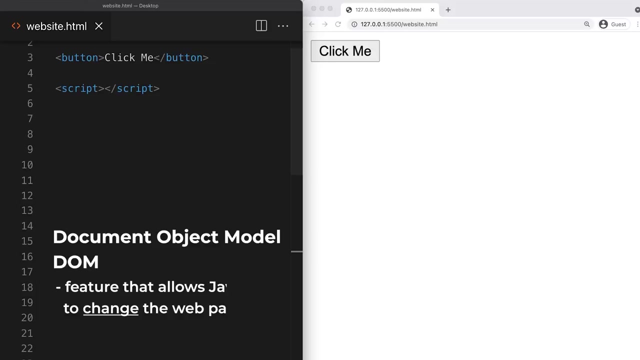 what makes our webpage interactive. so, for example, when we click something and type something, a bit of javascript code will update the page based on what we did. the most important feature of javascript is something called the document object model or the dom. the dom allows javascript to change the webpage. for example, this bit of javascript code uses the dom to change the text. 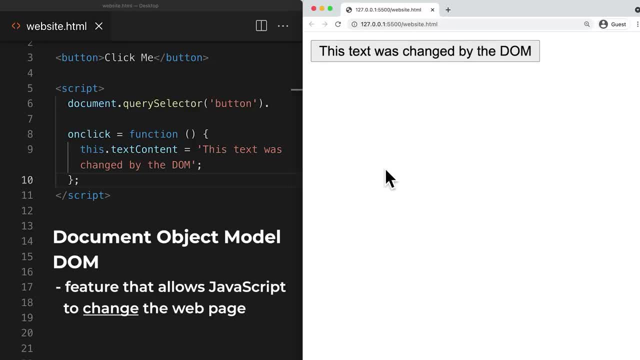 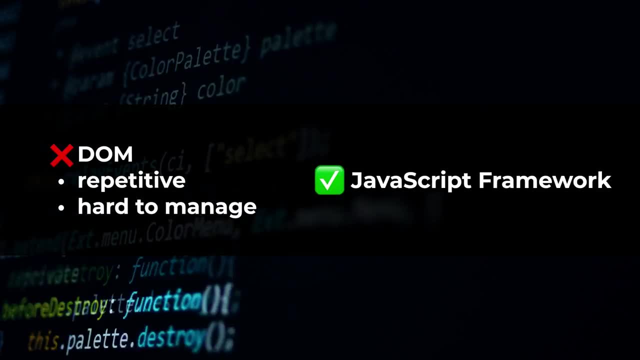 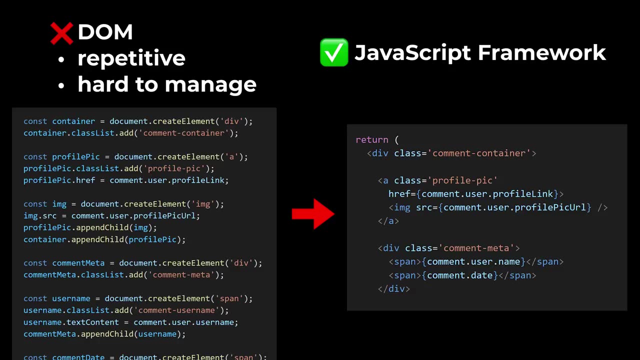 in the button, and this is how javascript makes pages interactive. however, using the dom directly like this is really repetitive and hard to manage, and that's why we use a javascript framework. javascript frameworks give us a much nicer way to create our webpage and they take care of updating. 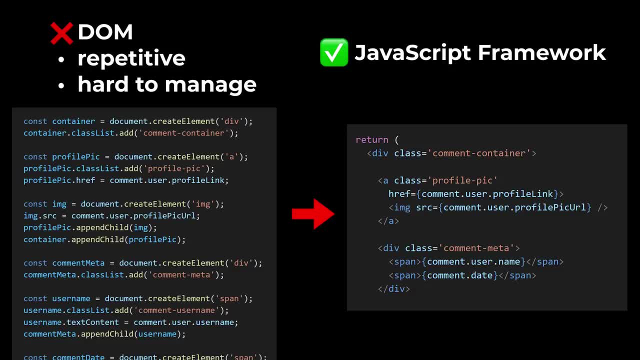 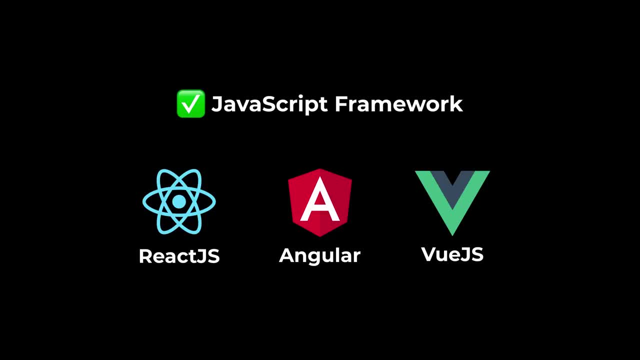 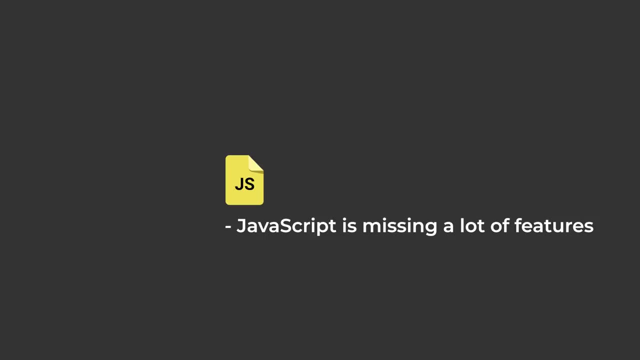 the page for us, so we never use the dom directly anymore. the most popular ones are reactjs and angular and vuejs. now let's take a step back and look at javascript again. javascript as a language is missing a lot of features that other programming languages have. one of these features: 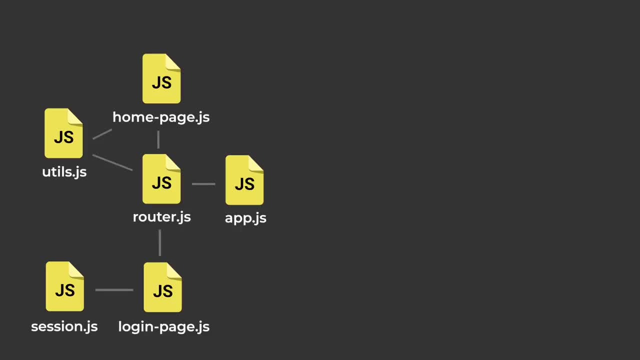 is being able to split up our code into different files and to organize our code. to solve this we have to use something called a bundler. the most popular one you've probably heard of is called webpack. webpack lets us split up our javascript code into many different files and once we're 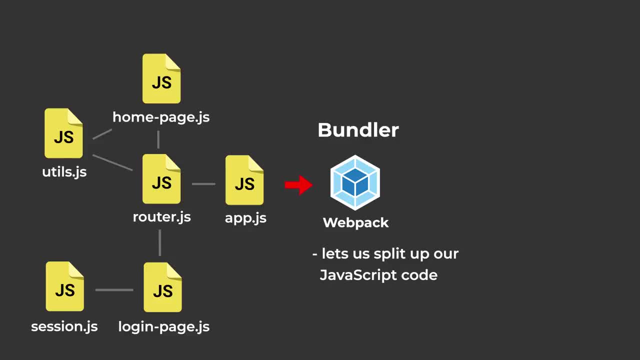 ready to put it on our website. webpack will combine all of these files or bundle all of these files into one javascript file that we can put on our website. another tool that we use is called a transpiler. the most popular one you've probably heard of is called typescript. 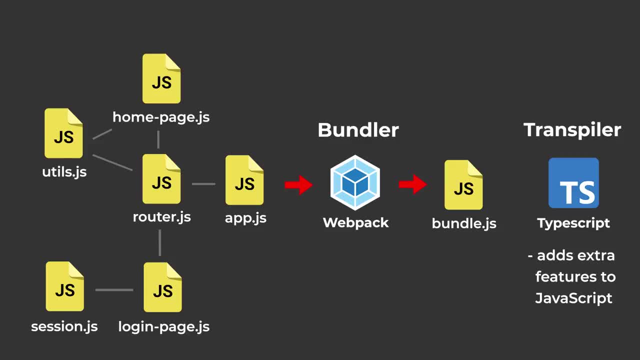 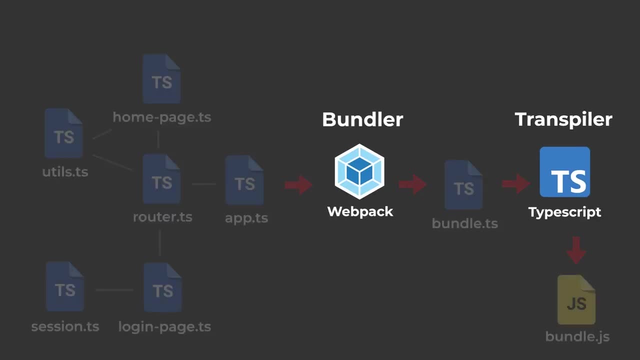 a transpiler adds extra features onto javascript. it lets us write an enhanced version of javascript and then, once we're done, it will transform the enhanced javascript back into normal javascript, because browsers like google chrome can only understand normal javascript. so those are the major technologies in the javascript world. now we're going to move over to css- css. 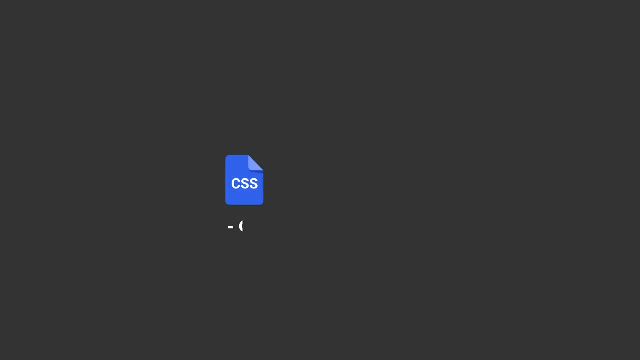 as a language has the same problems as javascript. we can't organize our code into different files, and css is missing a lot of useful features, so we also use a bundler and a transpiler for css. there's a special name for this, called a css pre-processor. 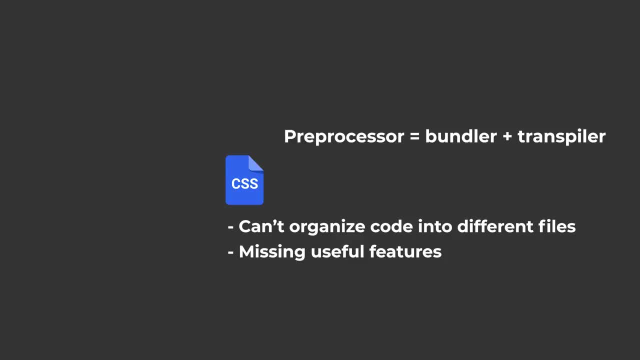 it's basically the combination of a bundler and a transpiler. the most popular css pre-processor you've probably heard of is called sass. sass lets us organize our css into different files and it lets us write enhanced css and then it will bundle all those files. 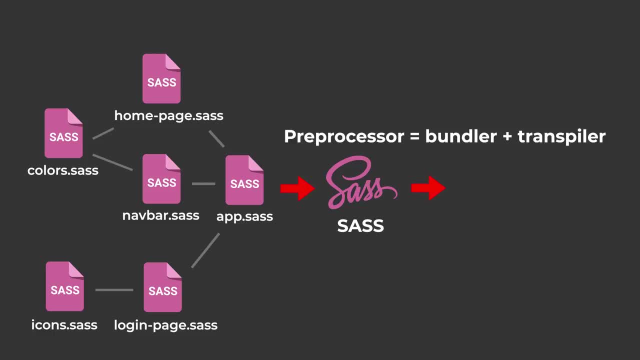 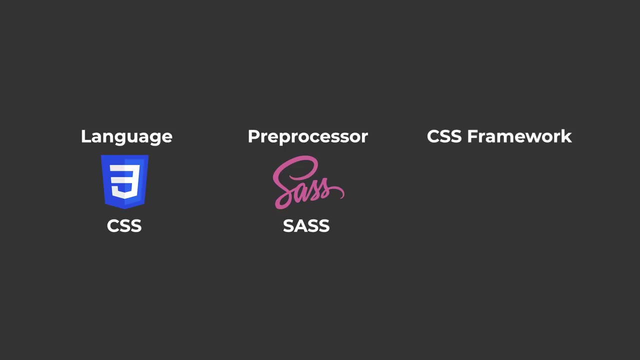 together into one file, and it will transform the enhanced css back into normal css, so you can think of it sort of like a bundler and a transpiler combined. now, once we had css preprocessors, developers start to create css frameworks, the most popular one being bootstrap. 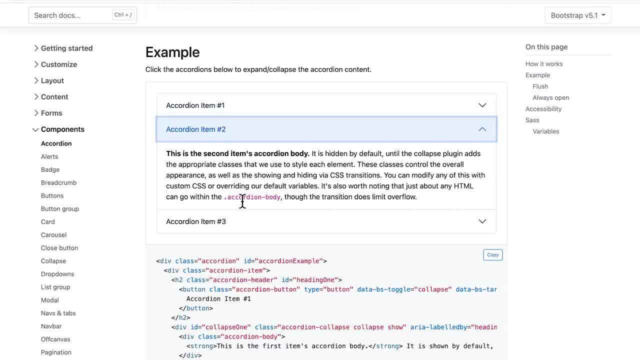 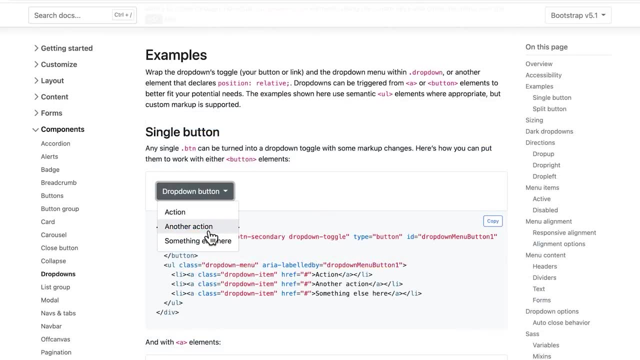 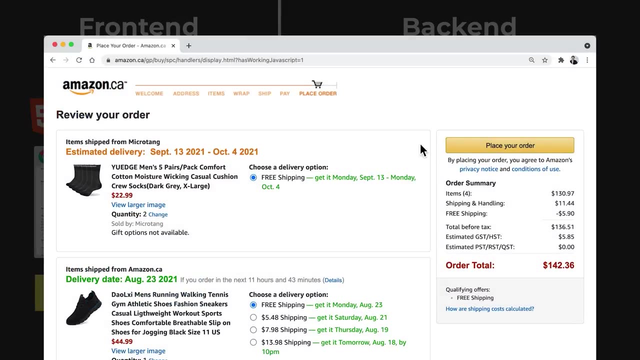 css frameworks are basically a whole bunch of css code that someone else wrote, and it helps us solve common problems, so using a framework like bootstrap saves us a lot of time. the last thing we're going to look at is how does the front end communicate with the back end. for example, let's say i'm on amazon and 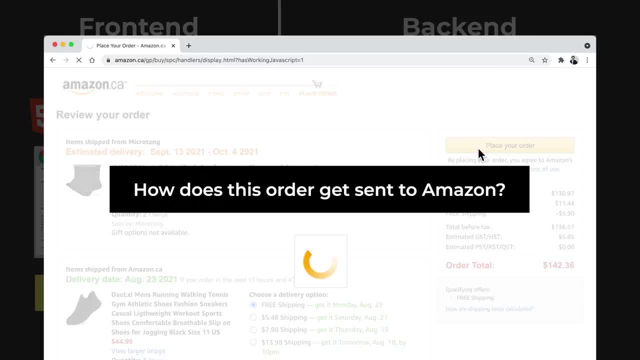 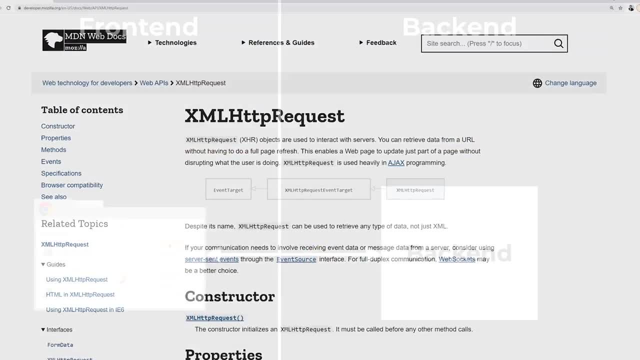 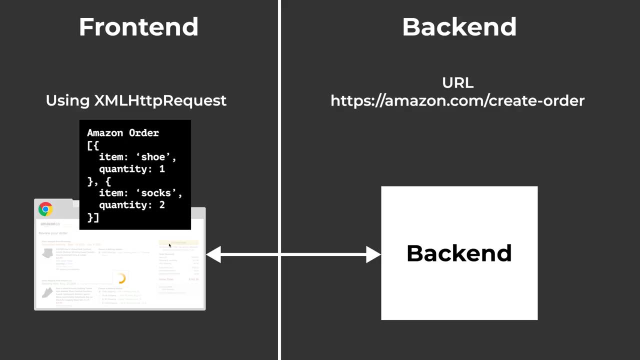 i want to make an order. how does this order get sent from my computer to amazon? javascript has a feature for this too: xml http request. it lets us send a message. in this case, we're going to send our amazon order to a url like amazoncom. create order on the other side.